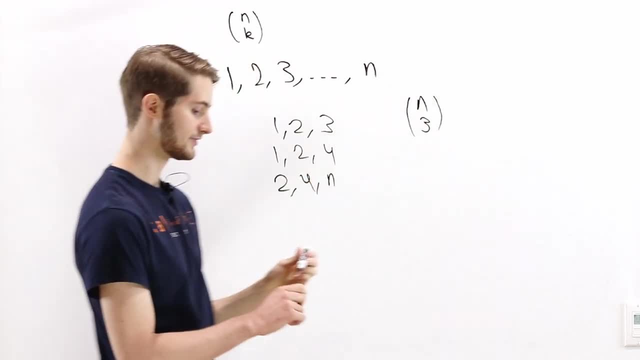 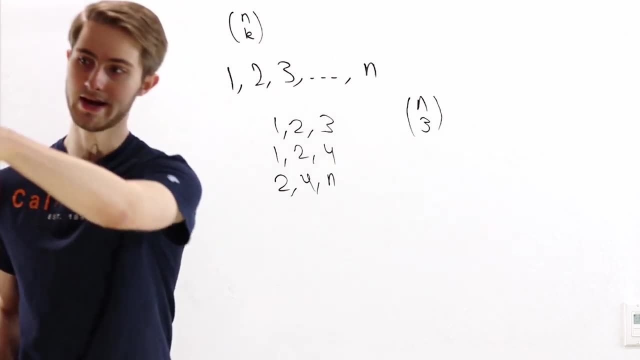 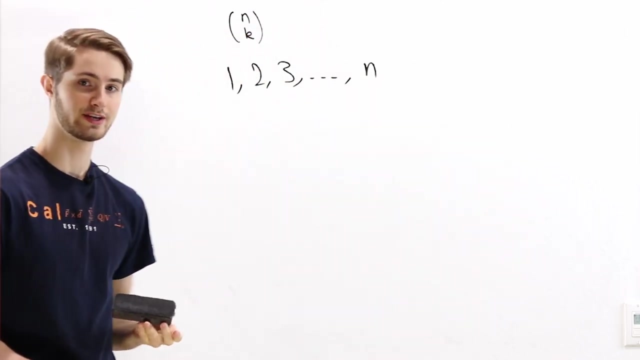 is called n choose 3, and it's denoted like this: More generally, the number of ways to choose k numbers out of n is denoted n choose k. In this video, I want to go through one of my favorite proofs for the formula for the value of n choose k, And in order to do that, we need to talk about: 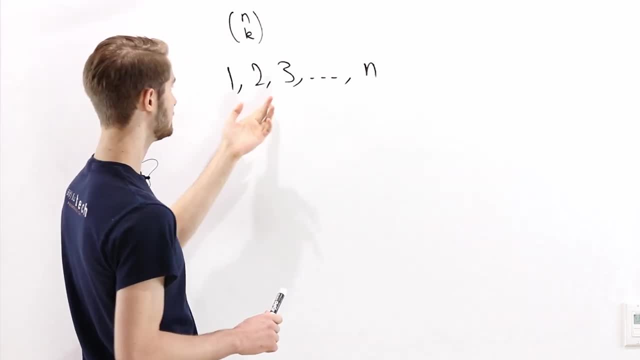 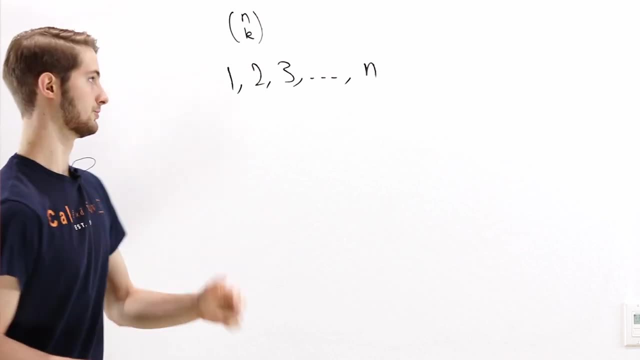 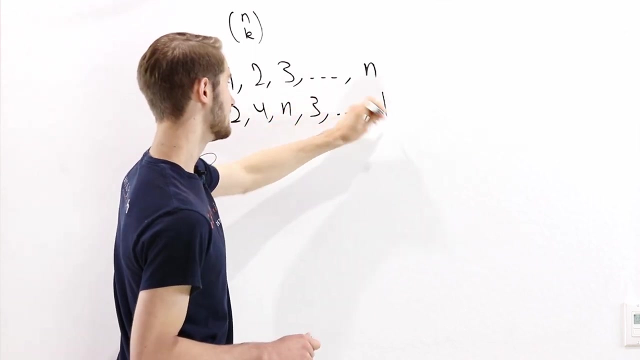 orderings. So here I have listed the numbers 1,, 2,, 3, and so on, up to n, and I've listed them in increasing order. But we could also write them in a different order. For example, I could write 2,, 4,, n, 3, and so on. 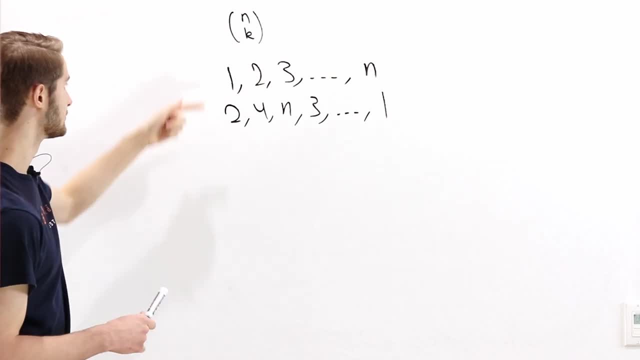 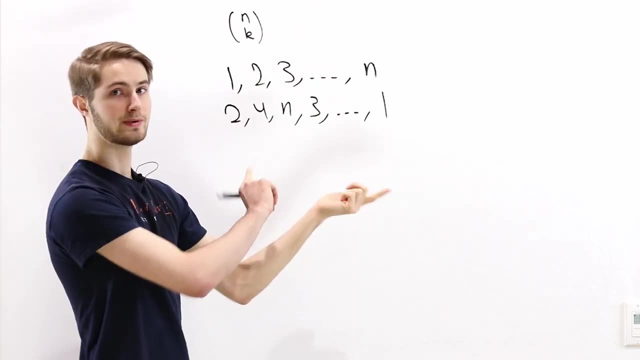 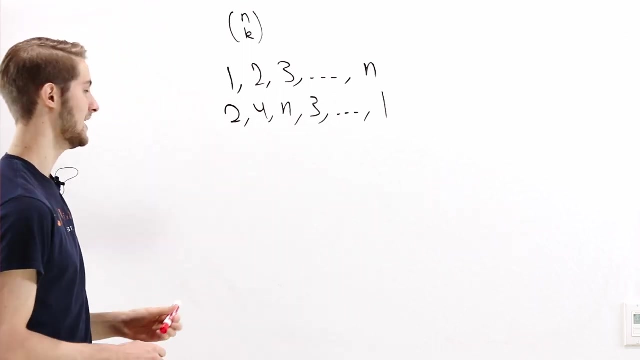 and then maybe the last number in the ordering is 1.. So both of these have the same numbers. it's just the numbers from 1 to n, except in this second line I've switched them around, so they're in a completely different order. Now, if we have this ordering of the numbers from 1 to n, 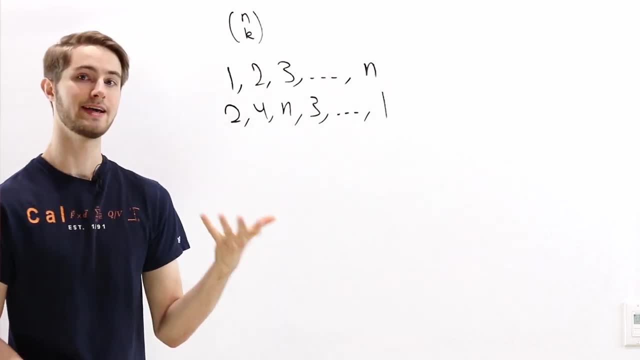 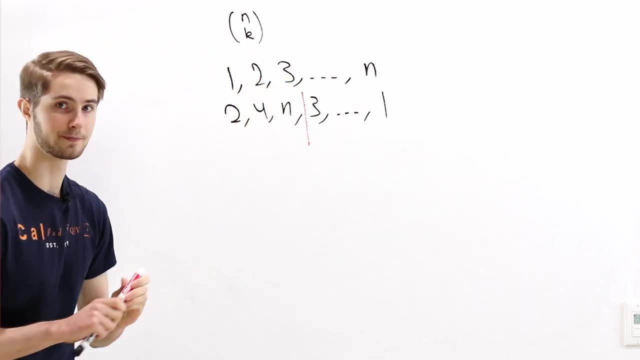 this ordering actually gives us a choice of k numbers, And the way that we do that is by just looking at the first k numbers in the ordering. So, like before, if we wanted to look at a choice of three numbers, we would look at the first three. 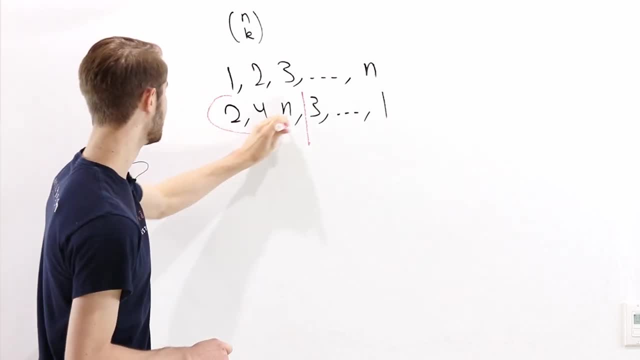 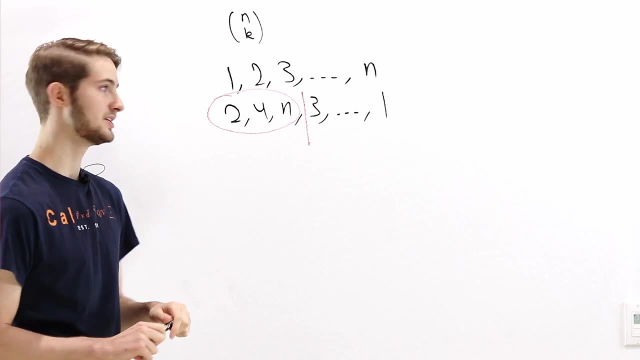 numbers in this ordering and we would get the choice of the numbers 2,, 4, n. So anytime we have an ordering of the numbers from 1 to n, whatever way we've switched them around, we can get a choice of k numbers out of n. 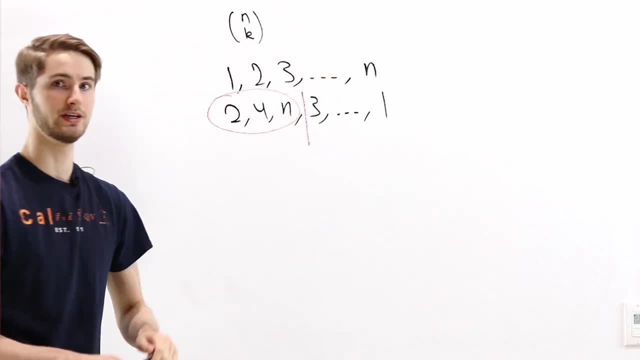 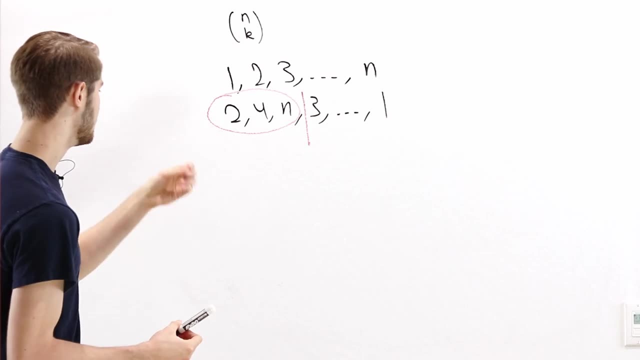 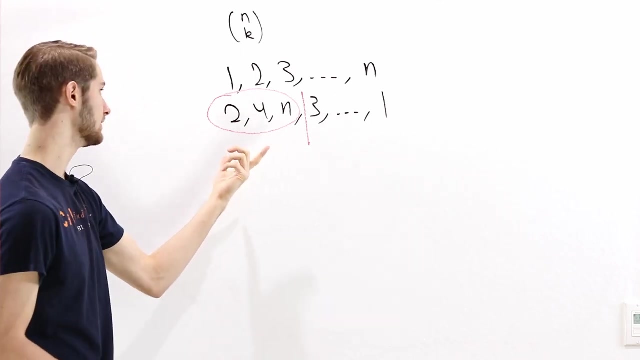 By looking at just the first k numbers in the list. And similarly, if we have any choice of k numbers out of n, we can put those k numbers at the front of a list and then that ordering gives us the choice of k numbers that we want. So if we started with the choice 2,, 4, n we could get. 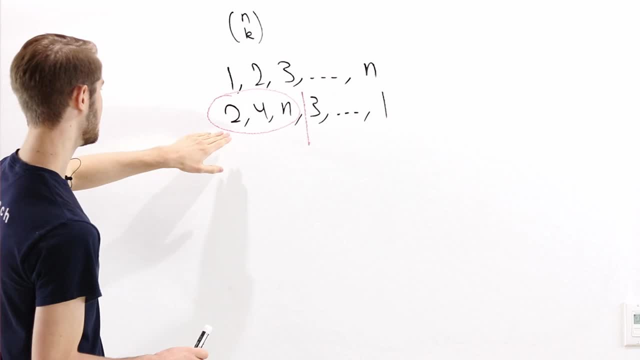 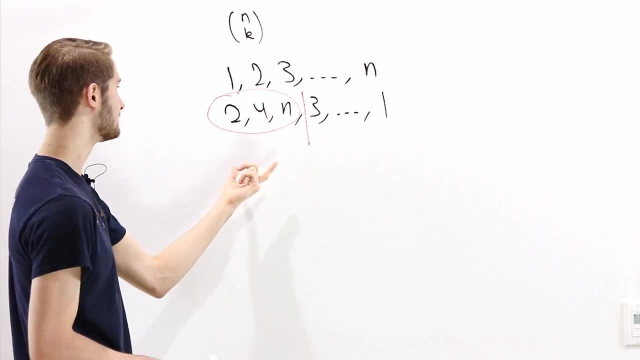 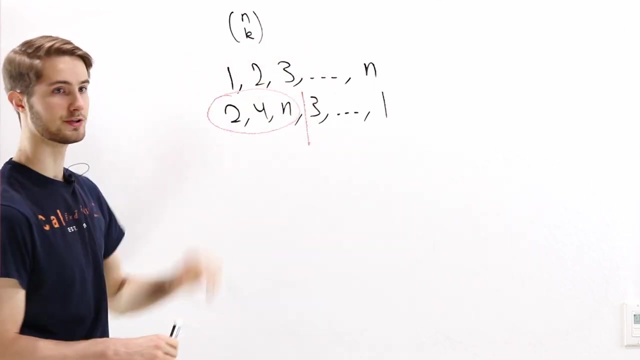 an ordering that gives us that choice by just putting 2,, 4, n at the start and then whatever we want at the end. It doesn't really matter, because it's just the start that we care about. So because of this fact, we can get every choice of k numbers from some ordering of the numbers 1 to. 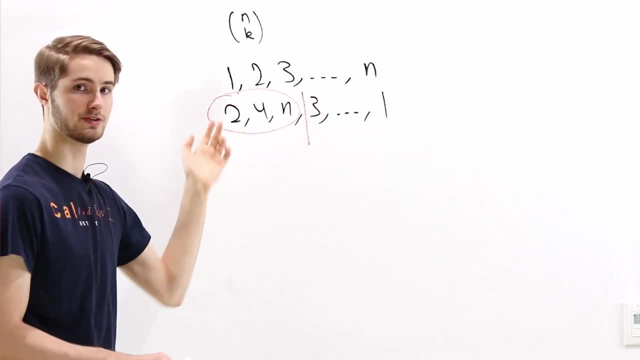 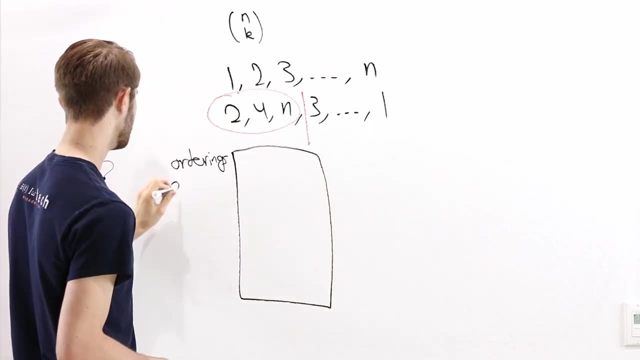 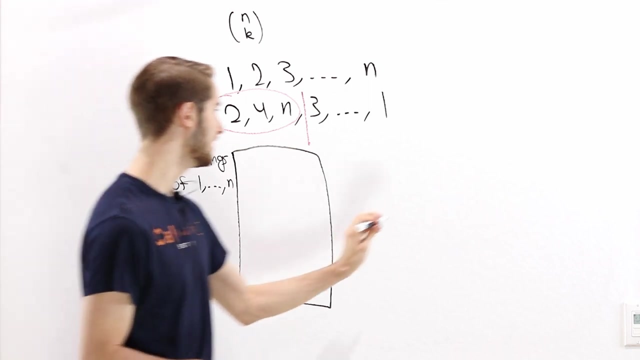 n, as long as we just put those k numbers at the front of the list. So let's think about the space right here of all orderings of the numbers 1 to n. So over here we have all of the orderings of the numbers from 1 to n. 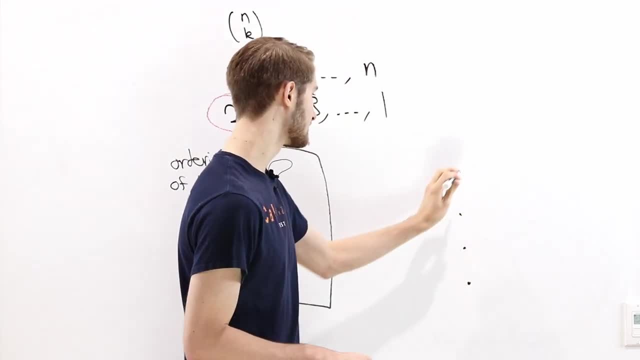 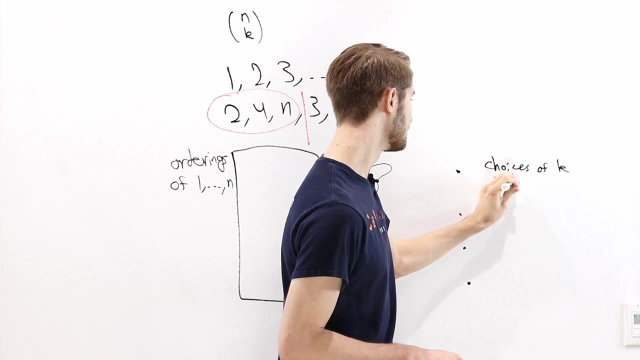 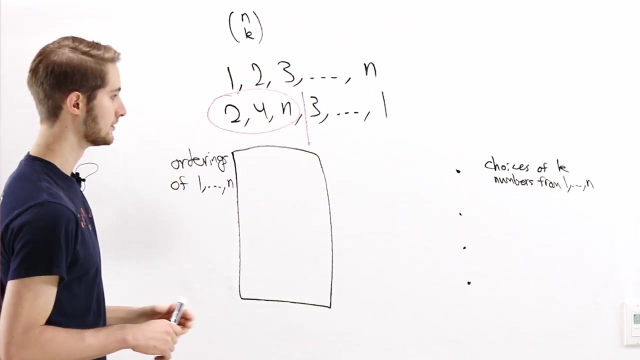 And then over here I'm going to put as dots these are all of the choices of k numbers from the numbers 1 to n. So the number of dots over here is the number of choices of k numbers from 1 to n, which is n. choose k. 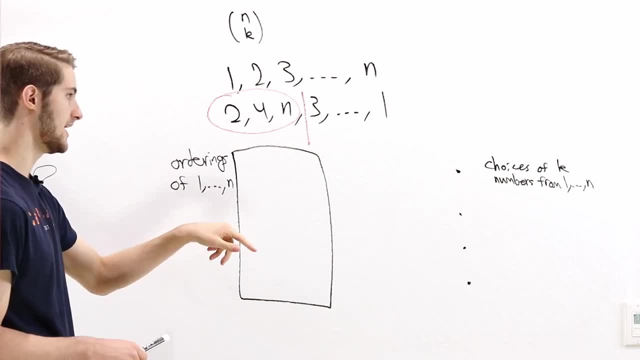 Now we said that, given an ordering of the numbers 1 to n, we can get an ordering of the numbers 1 to n which is n choose k. So we can get a choice of k numbers by looking at the first k numbers in that ordering. 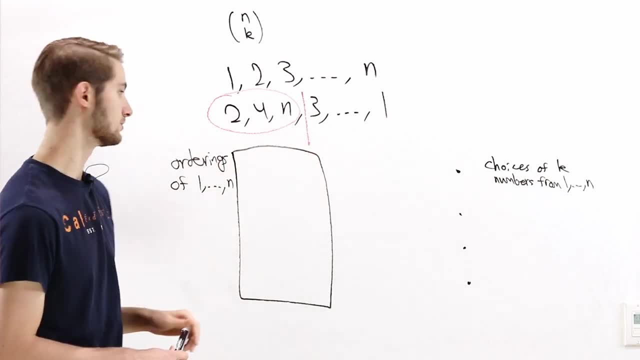 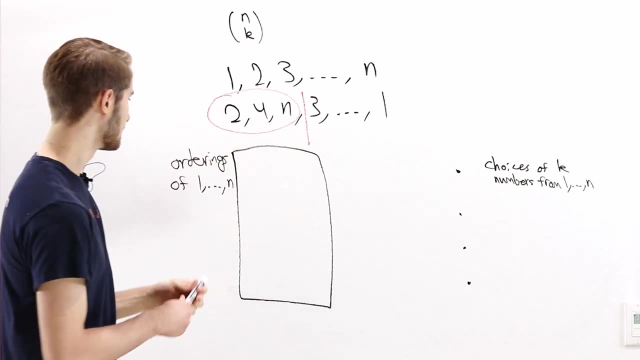 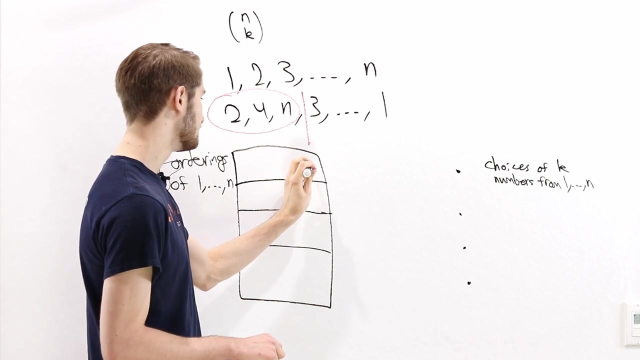 So if we have the space over here of all the possible orderings, we can split it up according to what are the first k numbers in the list. So I'm going to take this box and split it into some smaller boxes And we'll say that each one of these boxes, these smaller ones, 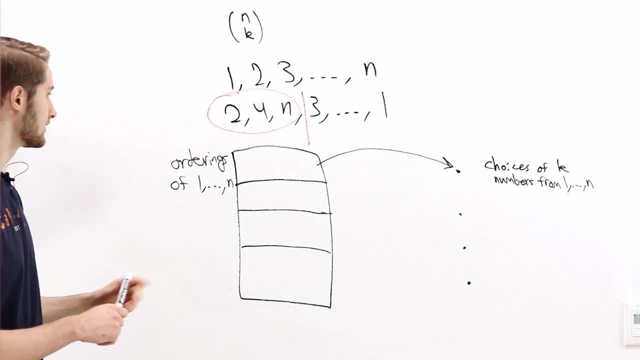 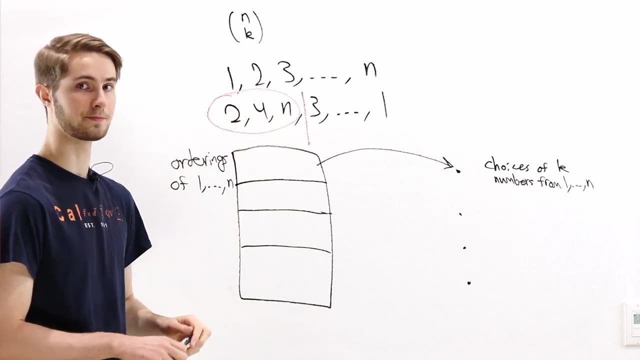 goes to a specific choice of k numbers. So within this box, every ordering in this box has the same k numbers at the start of the ordering. They might be flipped around a little bit but all of the k numbers at the start are the same for everything in this box. 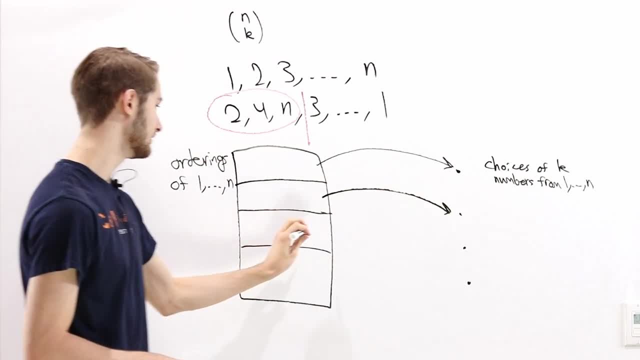 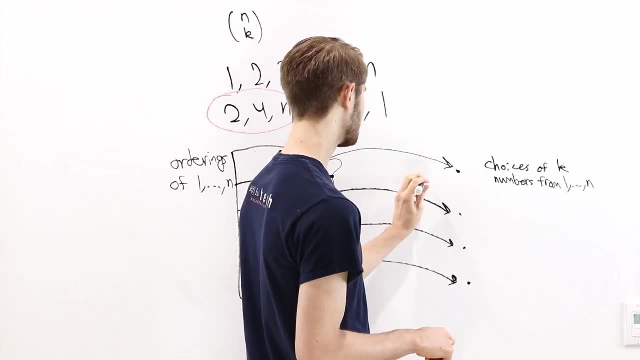 And similarly, this box is going to have a different choice of k numbers and so on. As an example, let's say that this dot right here corresponds to the choice of the numbers from 1 to k. So the way we choose k numbers is that we're going to have a choice of k numbers from 1 to n. 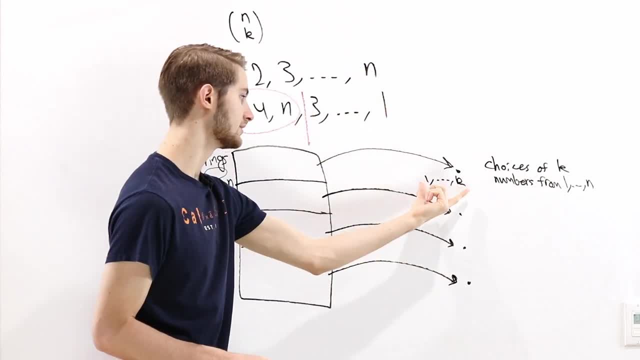 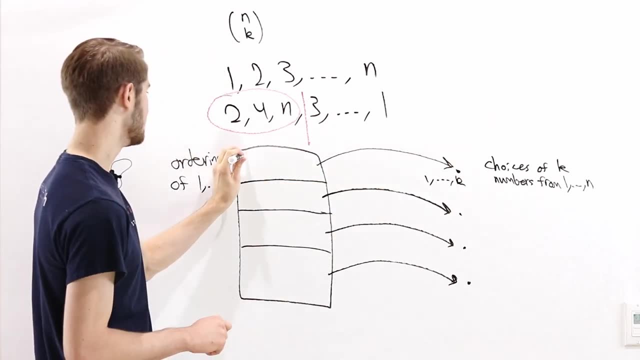 So the way we choose k numbers from the integers 1 to n is we just take the first k of them. One of the orderings of 1 to n that would go to this choice of k numbers is if we just took the integers from 1 to n in increasing order. 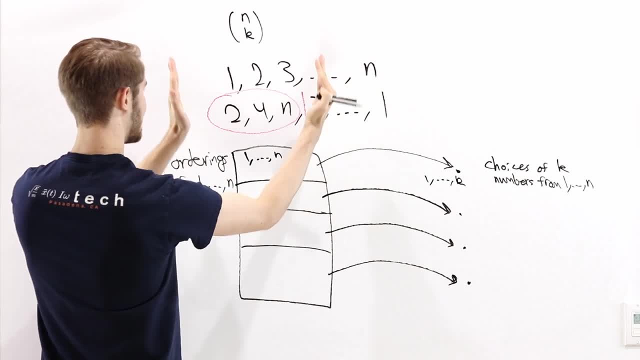 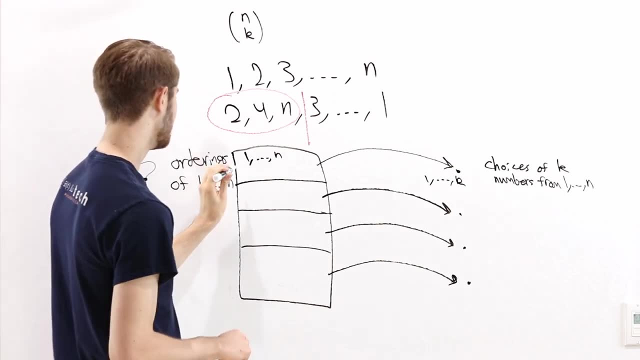 Because if we take this ordering and we cut off the first k numbers, that's just going to be 1,, 2,, 3, and so on up to k. But another option we could have is we go from k and then we do k minus 1,. 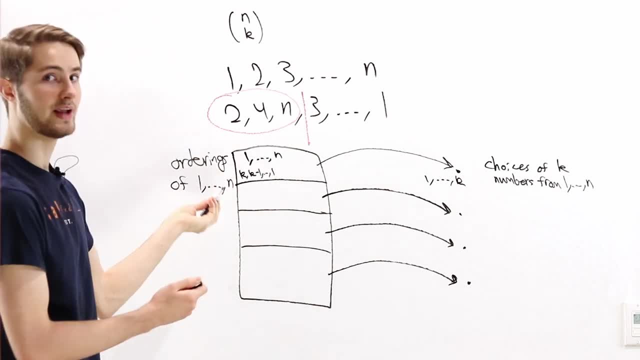 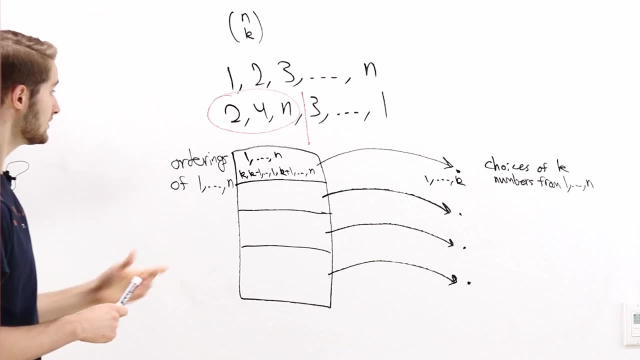 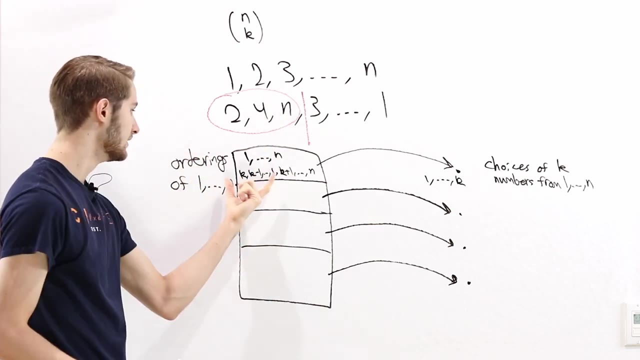 and then we do k minus 1.. And so on down to 1.. And then after that we do k plus 1, and so on up to n. So this is a different ordering of the first n numbers. But if we look at the first k, if we chop off the list right here, 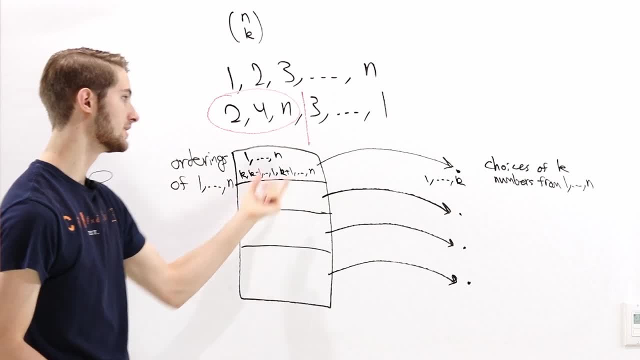 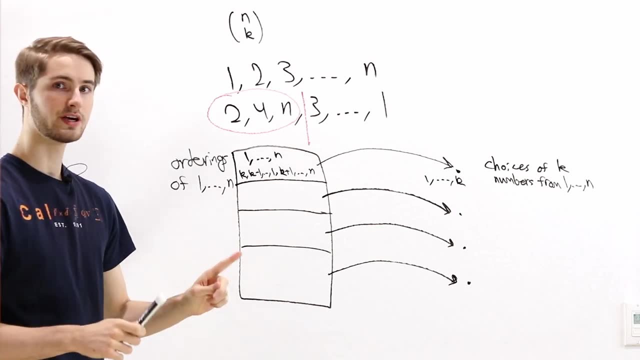 this is still all of the numbers from 1 to k, So this will still give us the same choice of k numbers, which means that these two orderings are going to be in the same box. Now the first thing I want to know is: 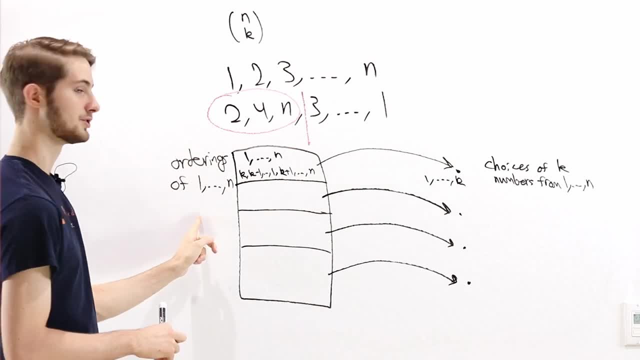 how many waves can we have in this box? How many waves can we order the numbers from 1 to n? How many orderings are there in total? Well, in order to get an ordering of the numbers from 1 to n, we can just think about picking each number in the list one by one. 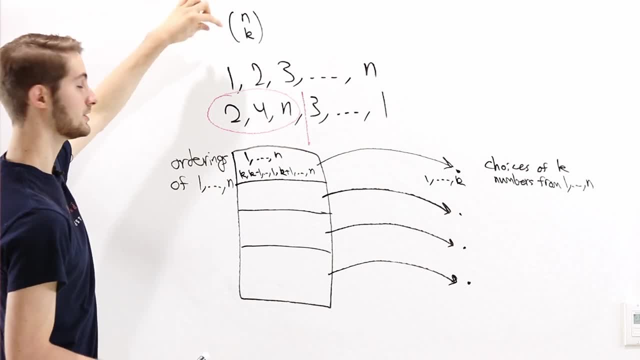 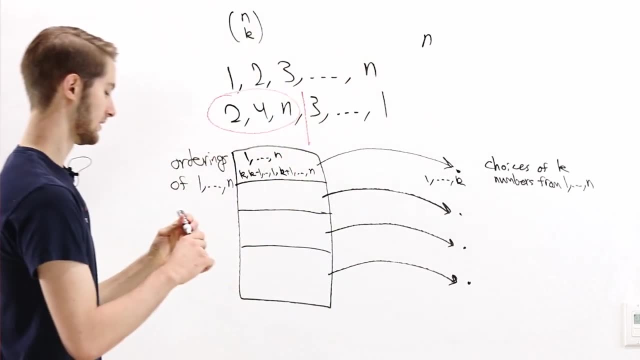 Since there are n numbers, if we start by picking the first number in the list, the number of choices we have for that first thing in the list is n. Now, after we pick something to go in the first slot, there are only n-1 numbers left. 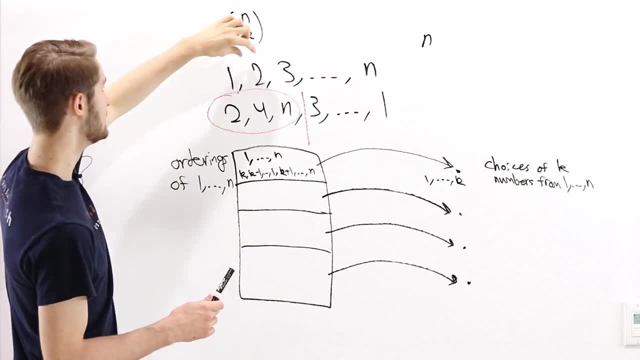 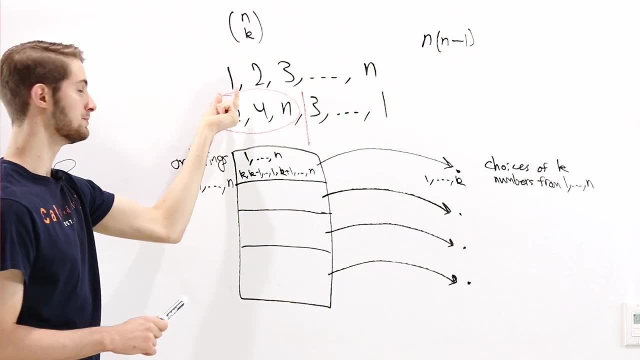 So after we pick something in the first slot, the number of choices we have left for the second slot is n-1.. It's all of the numbers except for whatever we put in the first slot. After that, when we go to the third one, 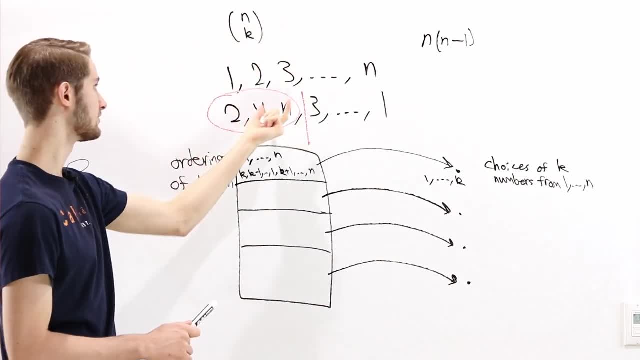 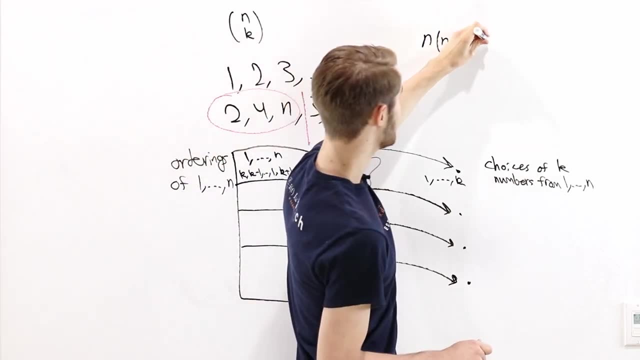 we've already used two numbers for the first two slots, so the number of choices here is n-2., And then after that it would be n-3,, and then so on, and we would go all the way down to 1.. 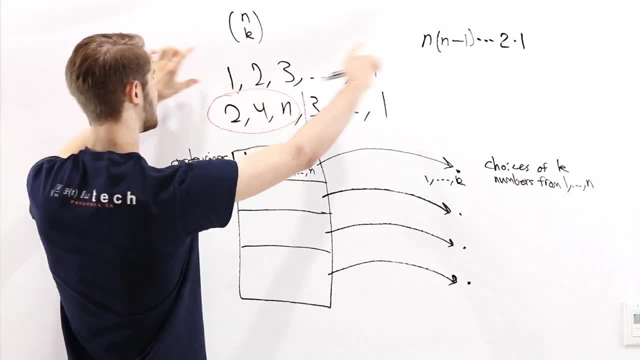 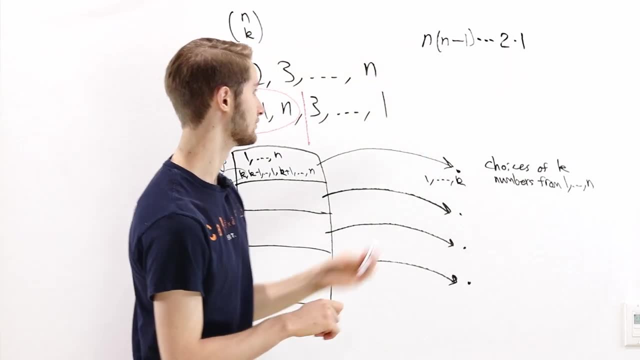 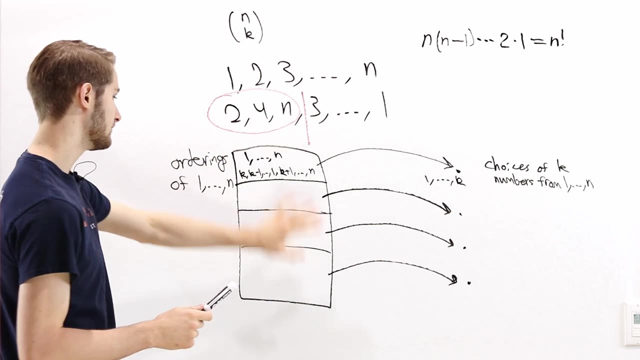 So the total number of choices we have for an ordering of these n numbers is going to be n times n-1, times n-2, and so on all the way down to 1, which is the same thing as n factorial. So the number of orderings in all these boxes together is n factorial. 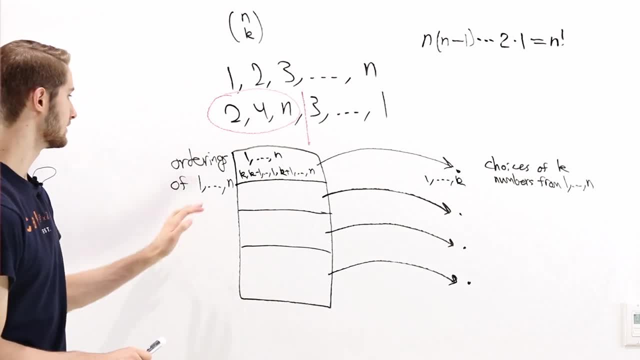 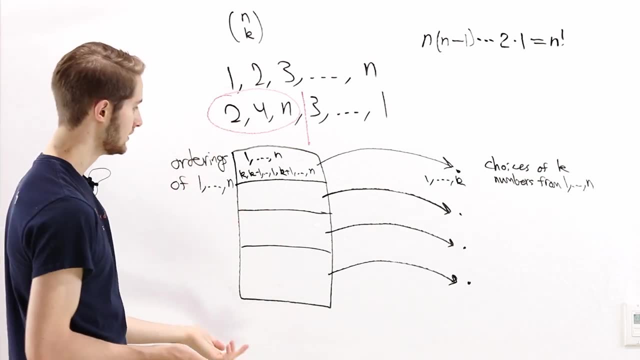 So now we know that the total number of orderings in all of the boxes is n factorial. But another way that we could find the number of orderings in all the boxes is to look at each of the individual boxes, find the number of orderings in those boxes. 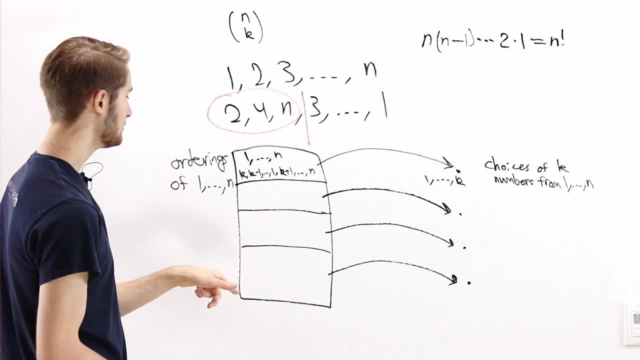 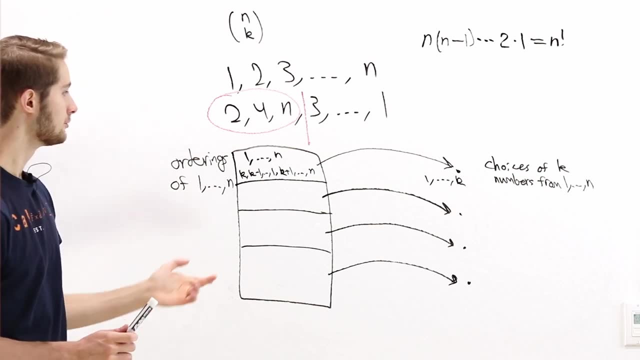 and then add them up. So now the question is: how many orderings are there in one specific box? Well, let's say we have some arbitrary box. We know that each box corresponds to a choice of k numbers, from the numbers 1 to n. 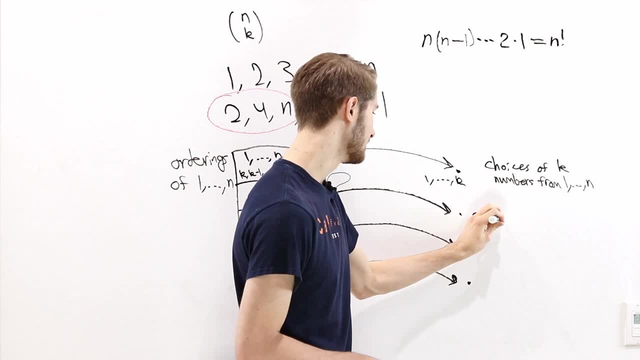 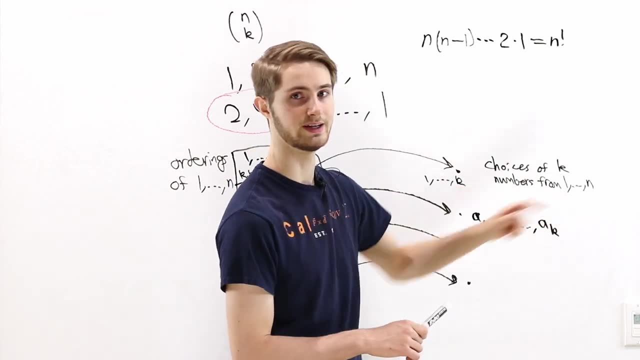 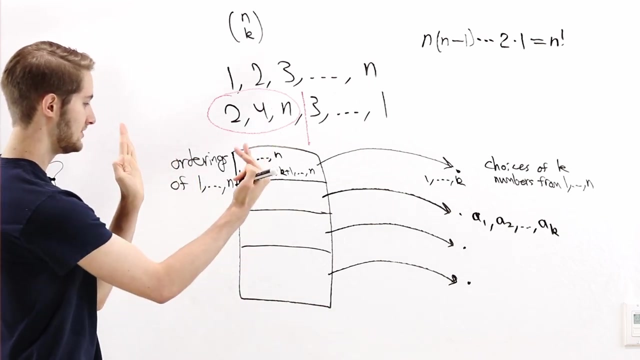 Let's say we have some arbitrary choice: a1,, a2, and so on up to ak. So these are just k numbers. These are just k whole numbers that are between 1 and n. Now everything in this box is an ordering where the first k numbers in that ordering. 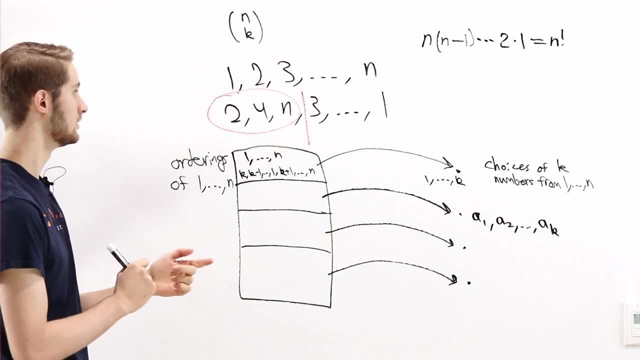 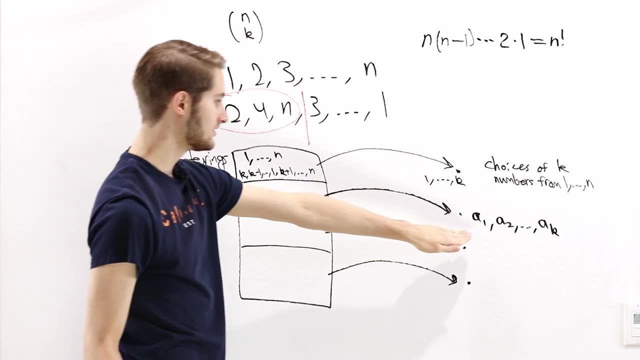 are these numbers in some order? We can flip them around. All that matters is that when we cut off the list at the point k right here and we look at everything to this side, it gives us a1,, a2, and so on to ak. 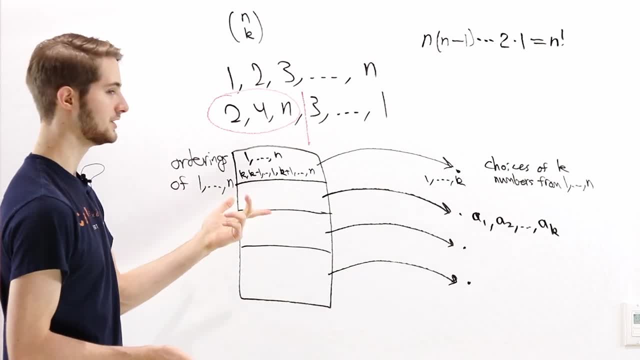 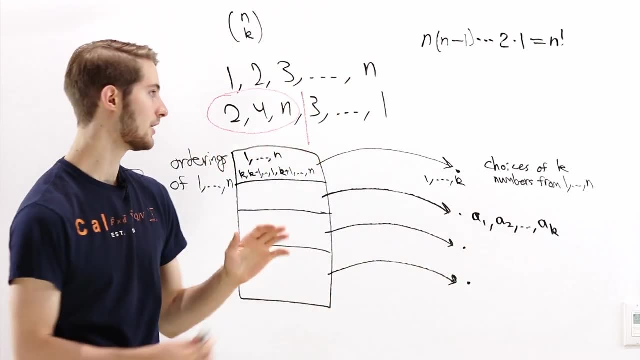 So if we want to know how many things are in this box, the question is, how many orderings are there that have a1, a2, and so on to ak as the first numbers out of those? n Well, if we wanted some ordering, 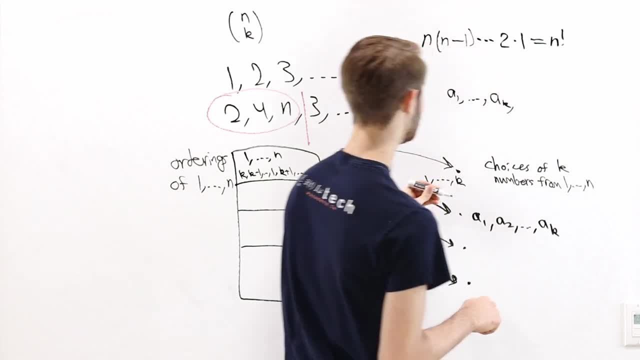 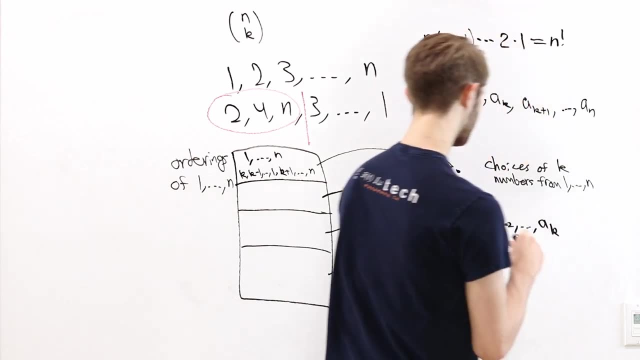 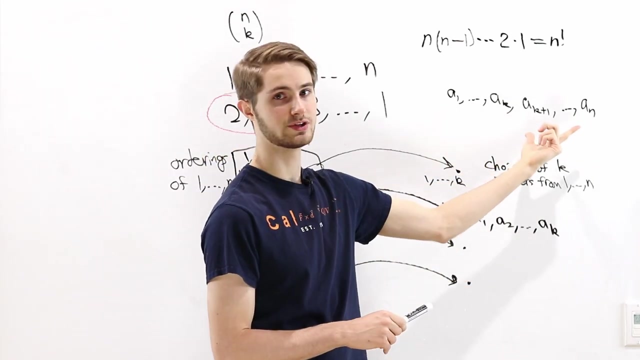 we could have a1 and so on to ak, and then let's say, the rest of the numbers are ak plus 1 and so on up to an. So these first k numbers are the ones that correspond to the choice for this box, and these are just the rest of the numbers, from 1 to n. 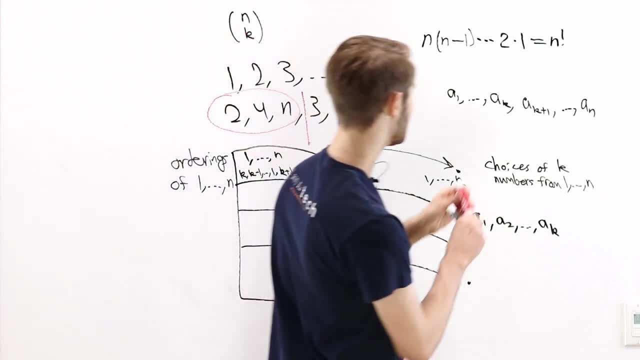 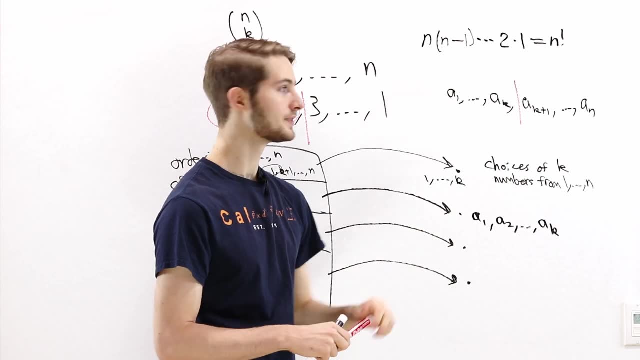 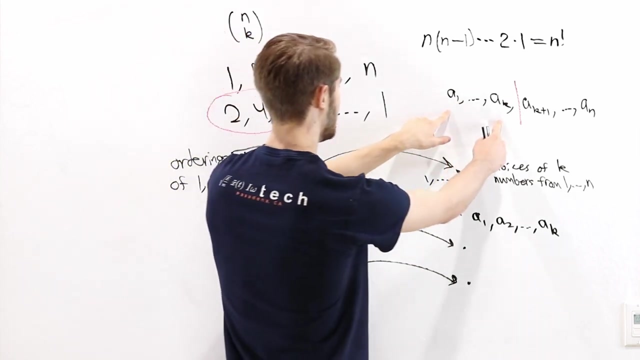 Now the important part is that when we cut off the list right here, any ordering that's in this box needs to have a1 to ak on this side of the line, But we can switch around the numbers on this side however we want. If we switch a1 and ak, 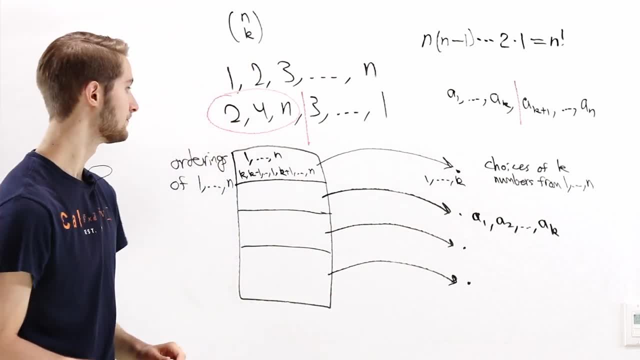 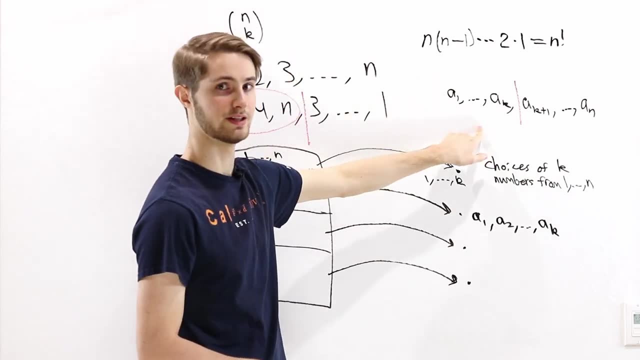 it's still going to give us the same choice of k numbers. So the orderings in here can have a1 to ak in any order that we want on this side of the line And if we look at the other side, ak plus 1 to an. 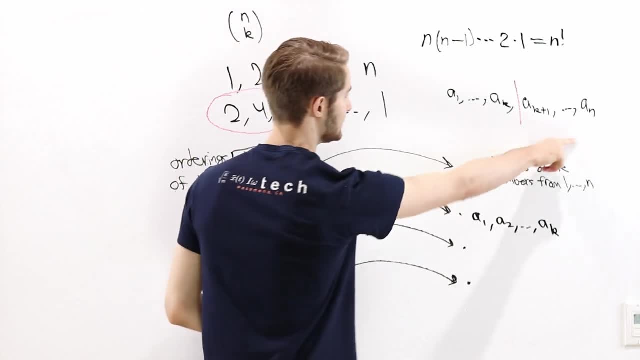 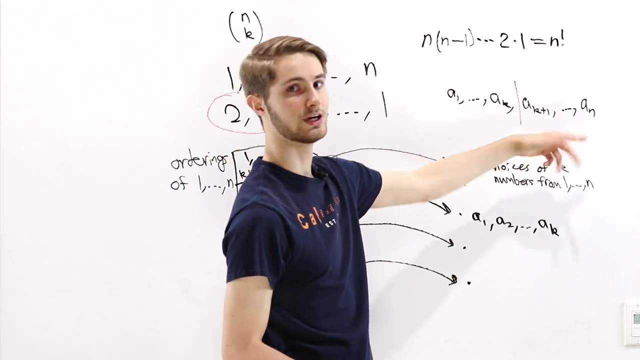 when we take the choice of k numbers, we ignore anything that's on this side of the line. These numbers just get thrown out because they're not in the choice. So we can flip these numbers around however we want as well, because they're going to get ignored anyway. 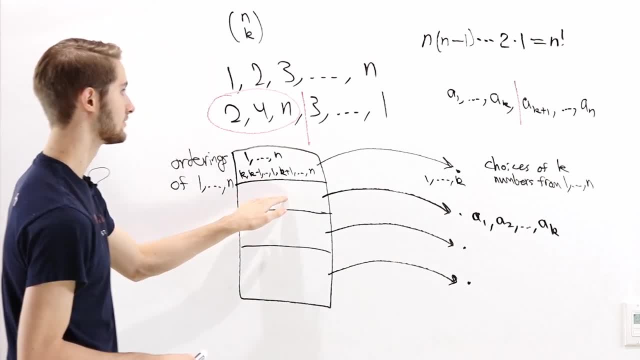 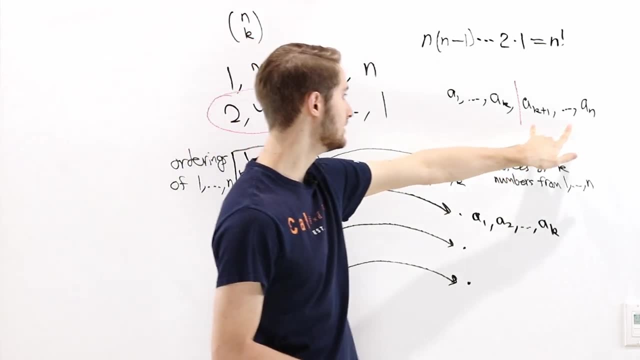 So if we want an ordering in this box, it's going to be the numbers from a1 to ak in any order on this side of the line, and then the numbers from ak plus 1 to an, in any order on the other side of the line. 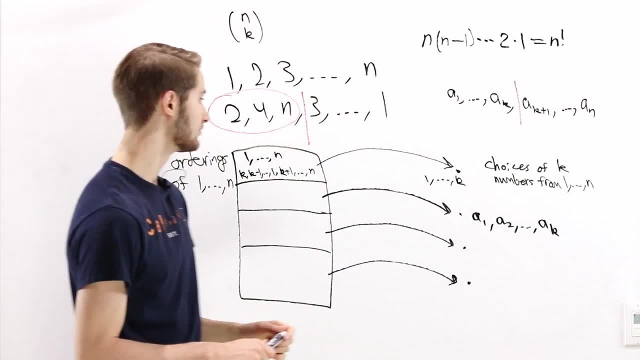 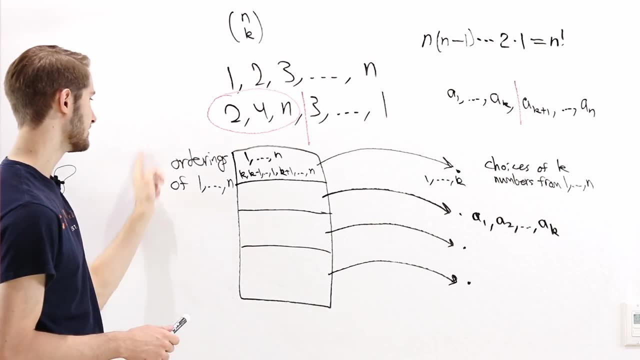 So how many ways are there to do that? Well, first we need to know the number of ways to order a1 to ak. But that's the same problem that we did earlier. We already found the number of orderings of the numbers from 1 to n. 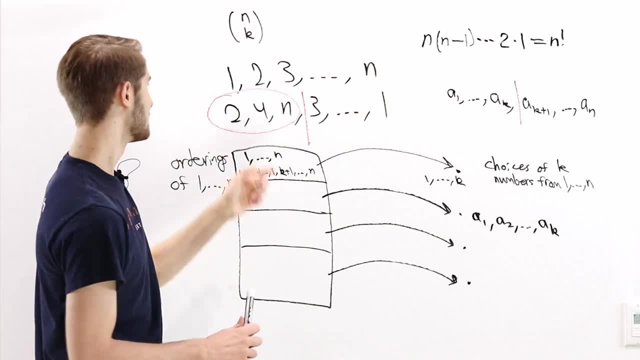 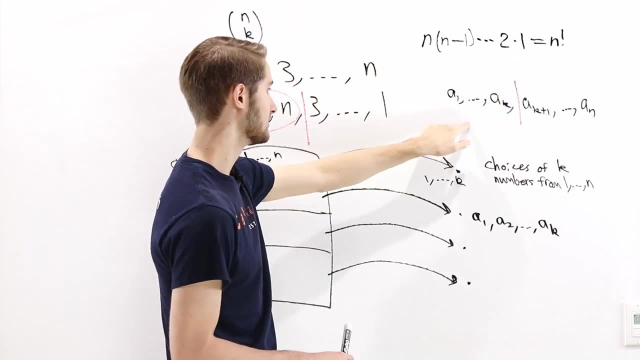 And that was just n- factorial, because there are n things, so we make n choices and that corresponds to the n numbers that we multiply here. So when we look at the numbers, the number of orderings of k things, it's going to be k factorial. 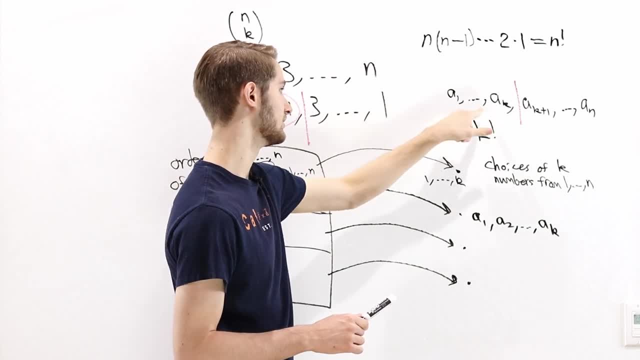 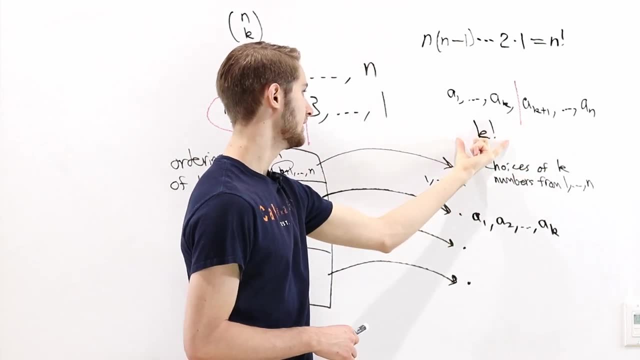 This is the number of ways that we can switch around these numbers: a1 to ak on this side of the line And over here. if there are k numbers on this side and there are n numbers in total, then over here there are n minus k numbers. 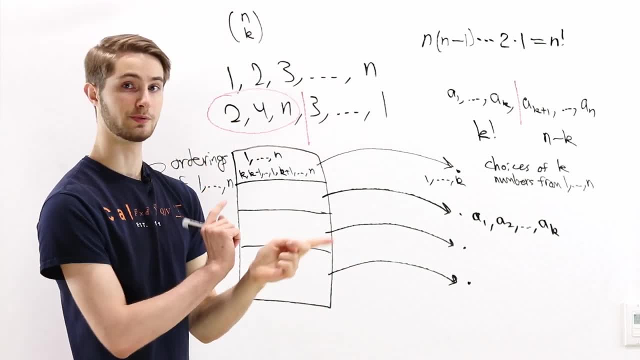 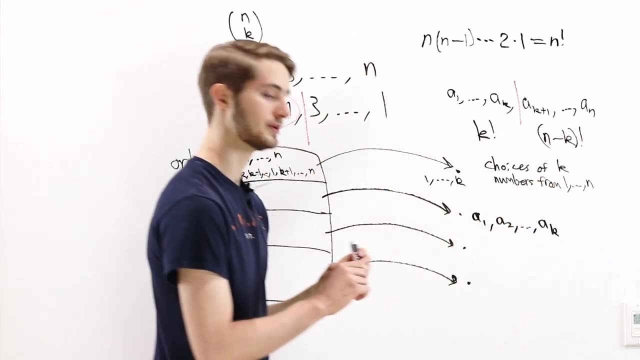 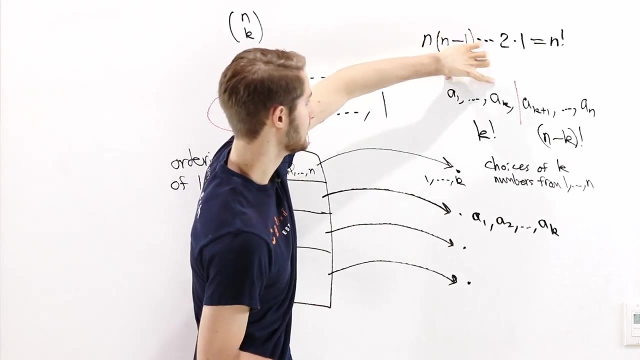 on this side of the line And we can order them however we want. The number of orderings for n minus k numbers is n minus k factorial by that exact same reasoning. So if we want an ordering in this box, we can have any ordering of the numbers a1 to ak. 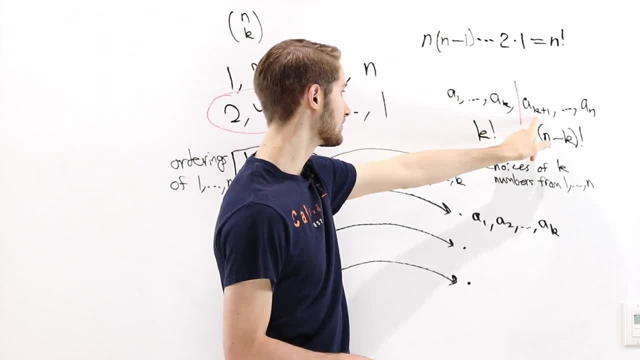 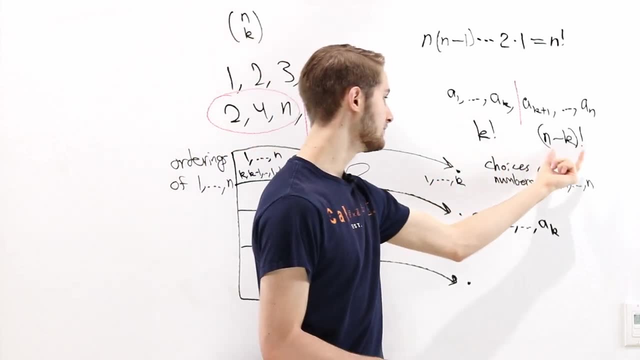 on this side of the line and we can have any ordering of the rest of the numbers on this side of the line. There are k factorial orderings on this side and n minus k factorial orderings on this side, So the total number of choices. 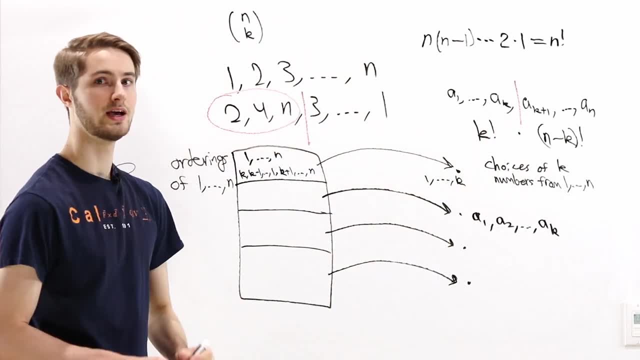 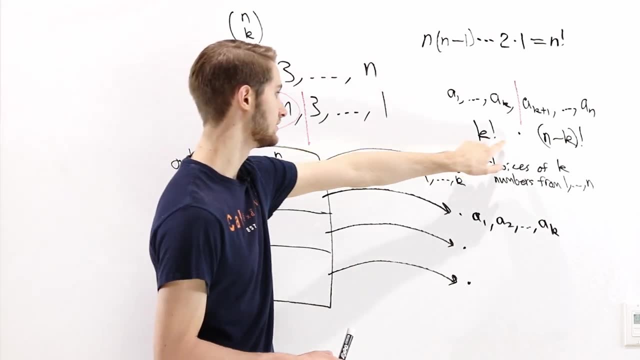 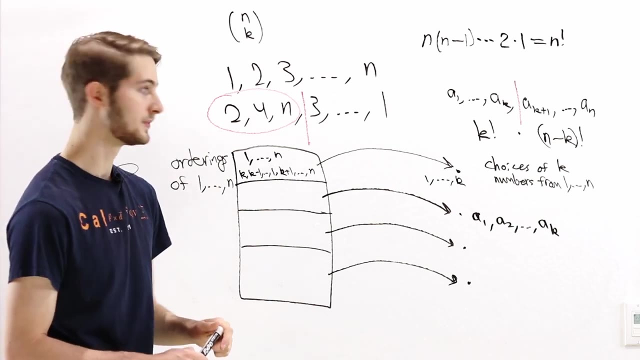 is going to be k factorial times n minus k factorial. So the number of things in each box is k factorial times n minus k factorial. The last thing we need to figure out is how many boxes are there? Well, each box corresponds to a choice. 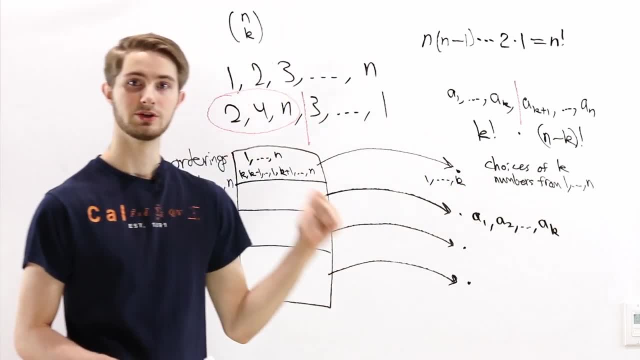 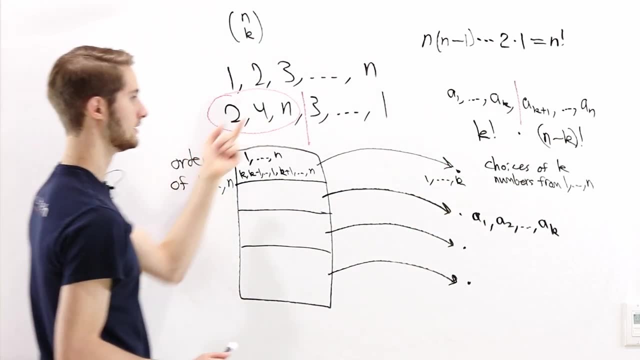 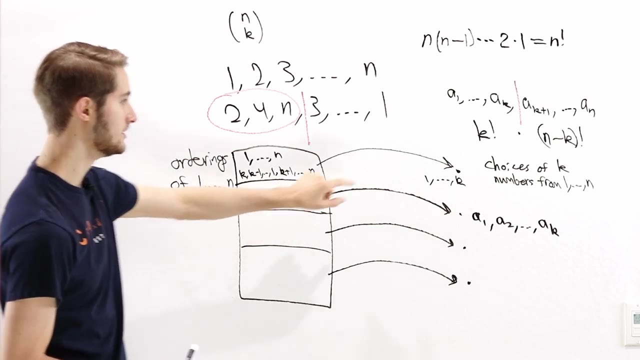 of k numbers from 1 to n And we showed earlier that every single choice of k numbers from 1 to n has some ordering that goes to that choice. So the number of boxes over here is the same as the number of choices of k numbers from 1 to n.